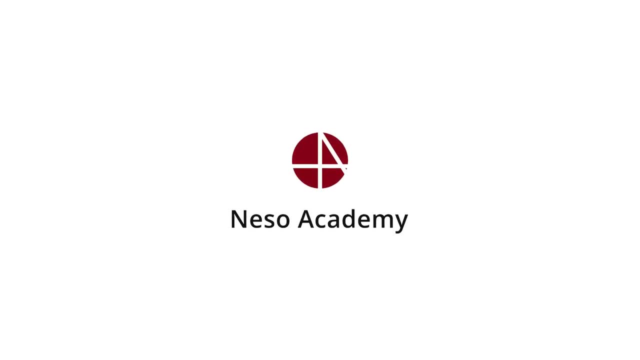 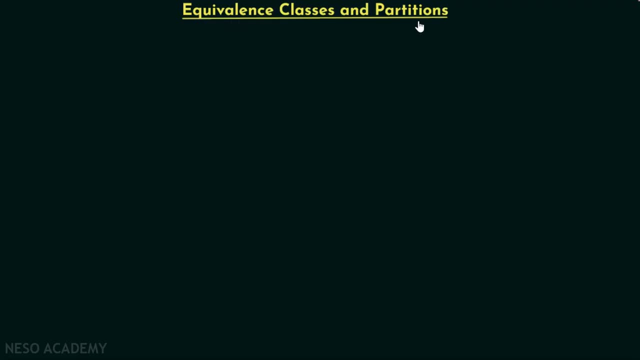 In this presentation we will discuss equivalence classes and partitions. So let's get started Here. we will discuss one theorem. Let R be an equivalence relation on a set A. Following statements for elements A and B of set A are equivalent. These statements are equivalent. 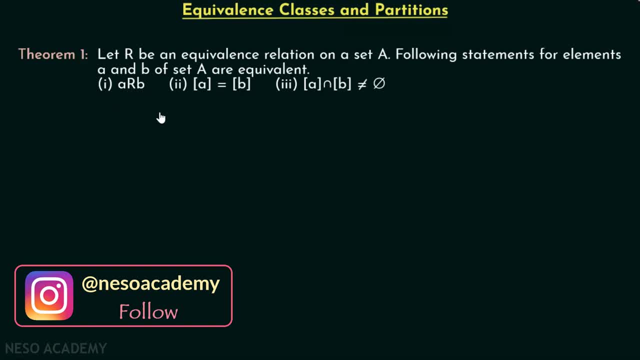 This is: according to this theorem, A is related to B. Equivalence class of A equal to equivalence class of B. Equivalence class of A: intersection equivalence class of B is not equal to phi. These three statements are equivalent. It must be well noted that R is an equivalence relation. 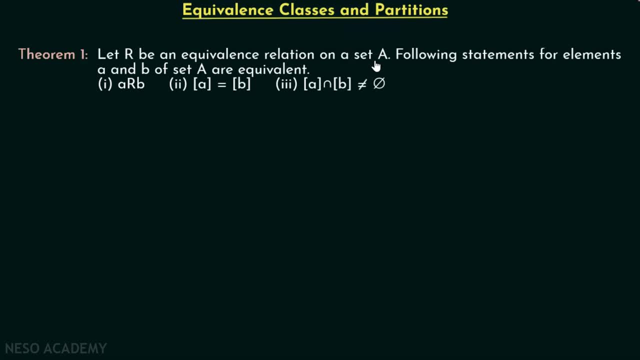 and this relation is defined on some set A. A and B are two elements of set A And for these two elements, these three statements are equivalent. Now we have to prove that these three statements are actually equivalent. Our target is to prove that 1,, 2 and 3,. 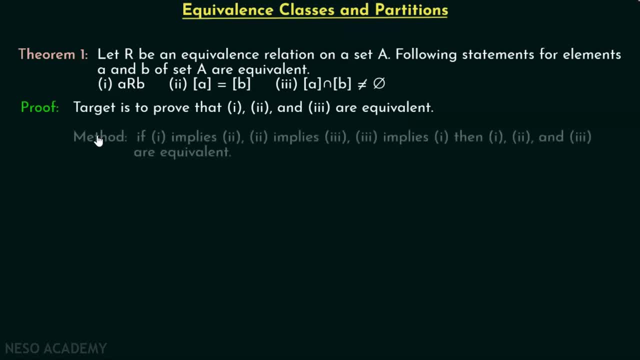 that is, these three statements are equivalent. Method is quite simple. If 1 implies 2,, 2 implies 3,, 3 implies 1,, then 1,, 2 and 3 are equivalent. It forms a kind of a cycle right. 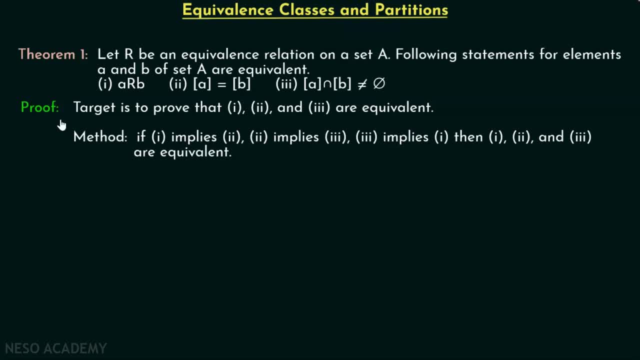 If 1 implies 2, 2 implies 3, 3 implies 1,, then obviously 1, 2 and 3 are equivalent. Let's first try to prove that 1 implies 2,, that is, when A is related to B. 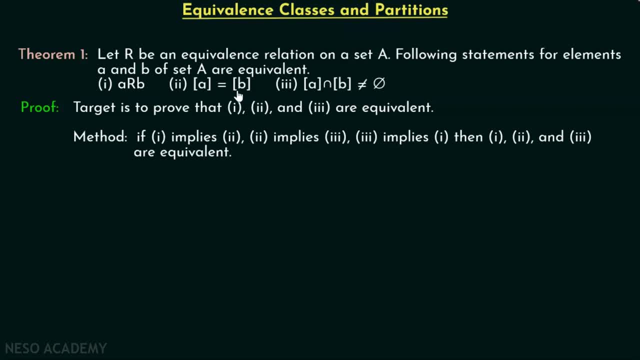 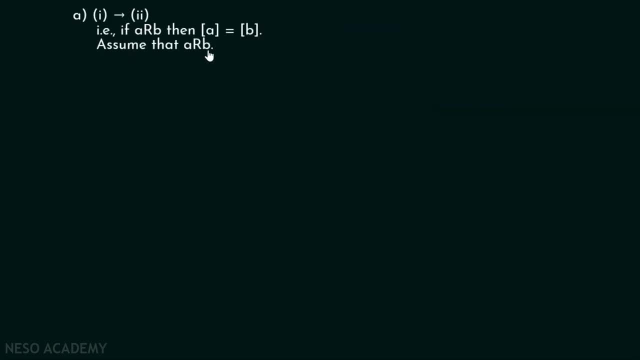 then equivalence class of A must be equal to equivalence class of B. Okay, Let's just try to prove this. For this, let us assume that A is related to B, Because it is given that if A is related to B, then equivalence class of A must be equal to equivalence class of B. 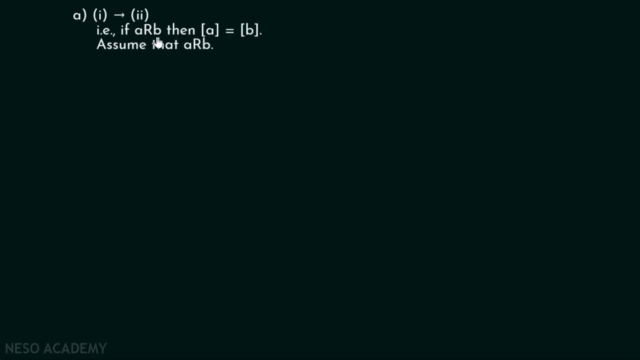 Right Here. we will first assume that A is related to B. Then we will try to prove that equivalence class of A is actually equal to equivalence class of B. We will now show that equivalence class of A is a subset of equivalence class of B. 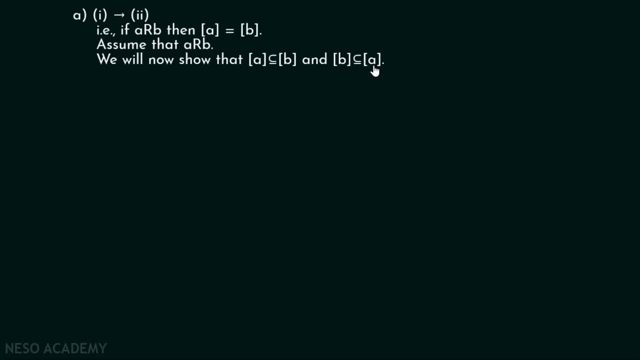 and equivalence class of B is a subset of equivalence class of A. For this, let's say that X belongs to equivalence class of A. Okay, Because we want to prove that equivalence class of A is actually a subset of equivalence class of B. 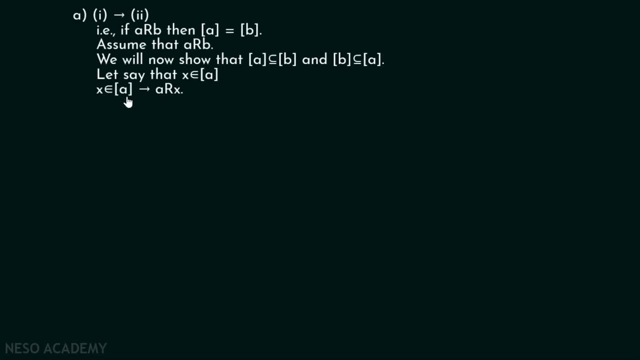 Right Here. if X belongs to equivalence class of A, then obviously A must be related to X, Because element A is related to X, it is already part of this equivalence class and X also belongs to this equivalence class. Therefore, it is clear that A is related to X. 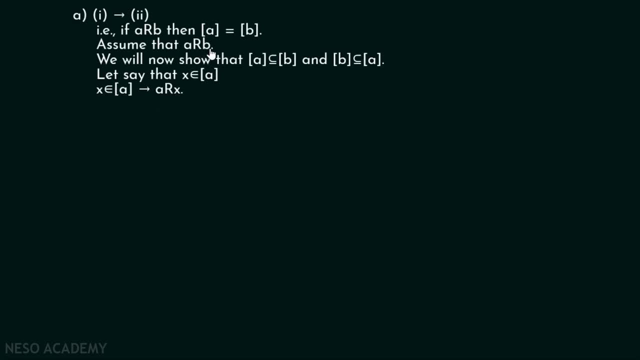 Right. We have assumed that A is related to B. This means B is related to A, Because R is an equivalence relation. we should remember that Right. Hence R is also symmetric If B is related to A and A is related to X. 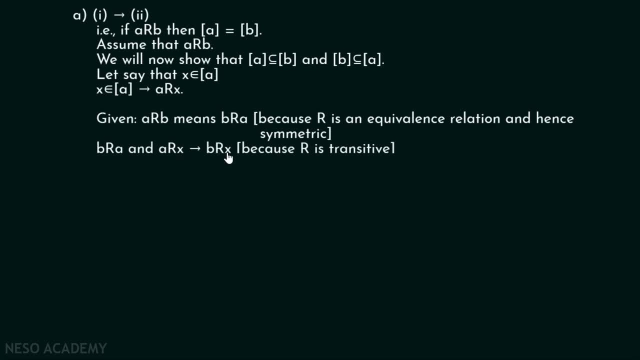 then B must be related to X. This is according to transitivity Right. If B is related to A and A is related to X, then obviously B must be related to X. Therefore X belongs to equivalence class of B According to this. 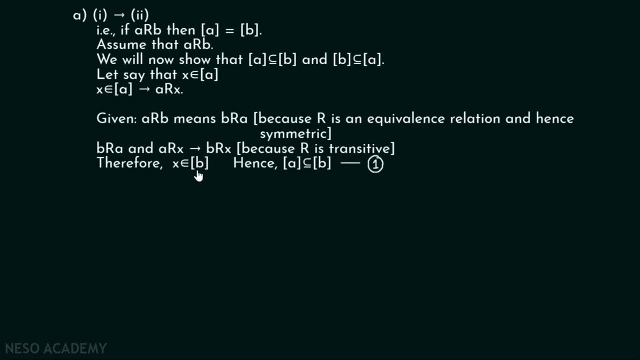 Right. B is related to X. This means that X must belong to equivalence class of B. Hence it is clear that equivalence class of A is actually a subset of equivalence class of B. Let's say this is one. Okay, Now let us assume that Y belongs to equivalence class of B. 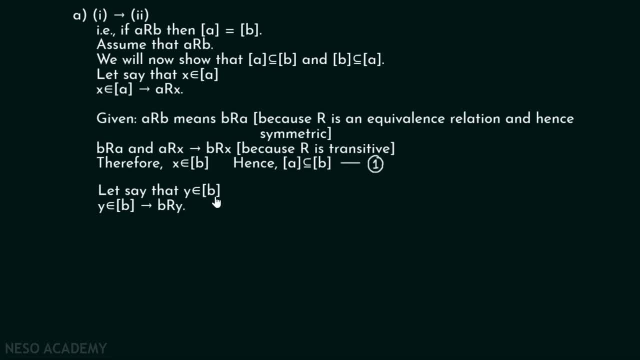 Some Y element belongs to this equivalence class. Now we want to prove the other side of the coin, That is, equivalence class of B must be the subset of equivalence class of A. Then only we would be able to prove that equivalence class of A. 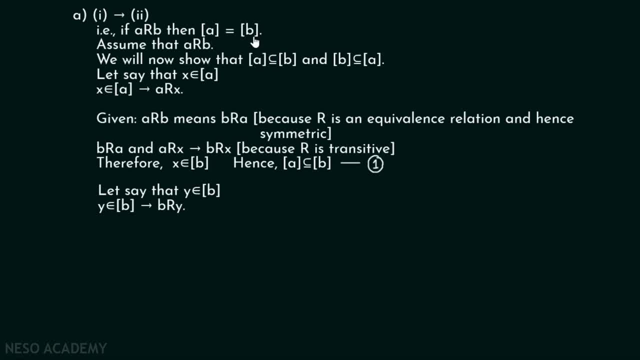 is actually equal to equivalence class of B, Right? That is why I am assuming here that Y belongs to B And Y belongs to equivalence class of B implies B is related to Y. There is no doubt about this. We have assumed that A is related to B. 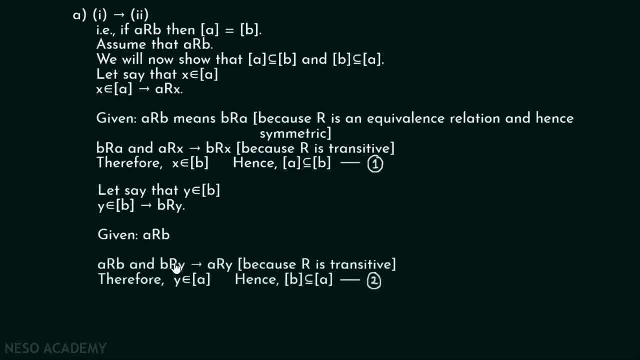 Now we know that A is related to B And B is related to Y. Therefore we can say A is related to Y. This is according to transitive property. Therefore Y belongs to equivalence class of A. Hence we can say that equivalence class of B. 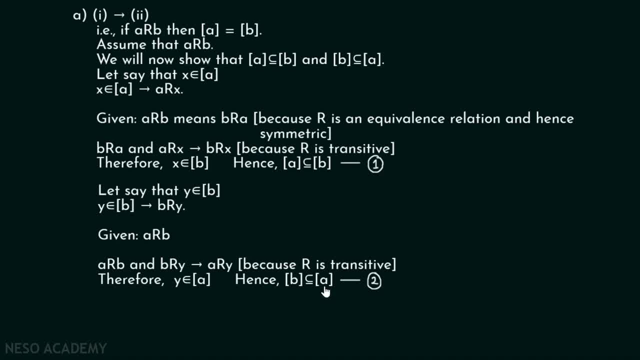 is a subset of equivalence class of A. Let's say, this is two From one and two. we can say that equivalence class of A is actually equal to equivalence class of B, Isn't that so? So this means that if A is related to B, 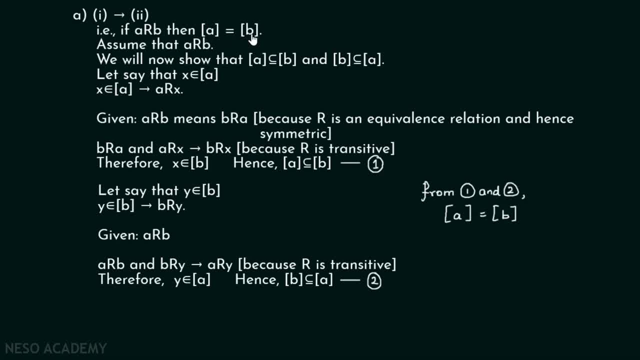 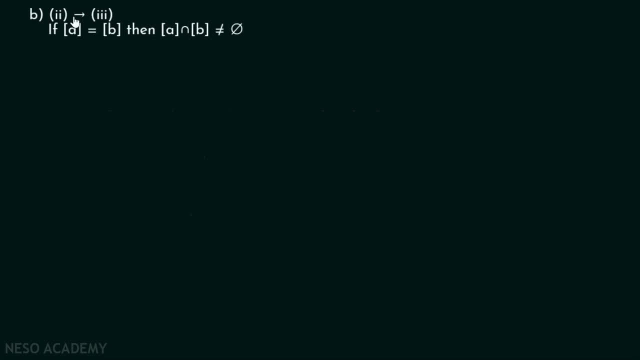 then equivalence class of A is actually equal to equivalence class of B. Therefore, one implies two. Now let's just try to prove that two is related to three. This means that if equivalence class of A is equal to equivalence class of B, 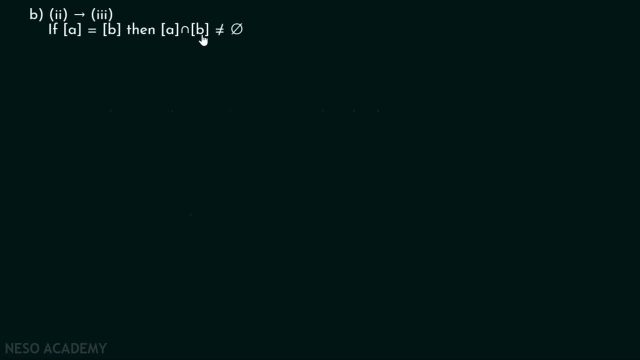 then equivalence class of A intersection equivalence class of B must not be equal to five. That's what we want to show. Let us assume that equivalence class of A is actually equal to equivalence class of B, Then obviously, equivalence class of A intersection equivalence class of B. 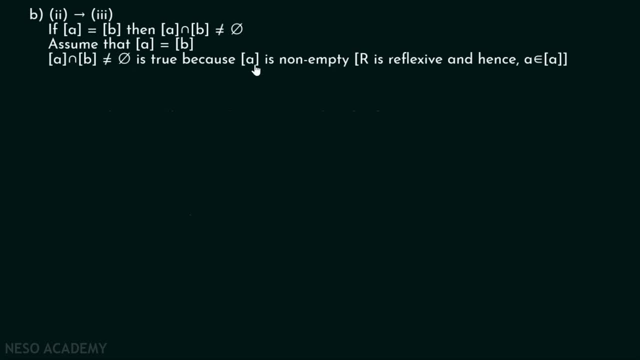 must not be equal to five, Because equivalence class of A is non-empty. We can replace this equivalence class of B by equivalence class of A. Then this becomes equivalence class of A, intersection equivalence class of A. Obviously, this cannot be five right. 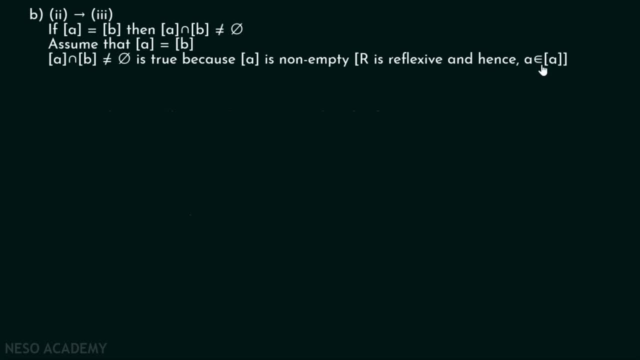 Because R is reflexive and hence A must belong to equivalence class of A, This element must belong to equivalence class of A. This means that equivalence class of A- intersection equivalence class of B- must not be equal to phi. Hence 2 implies 3.. 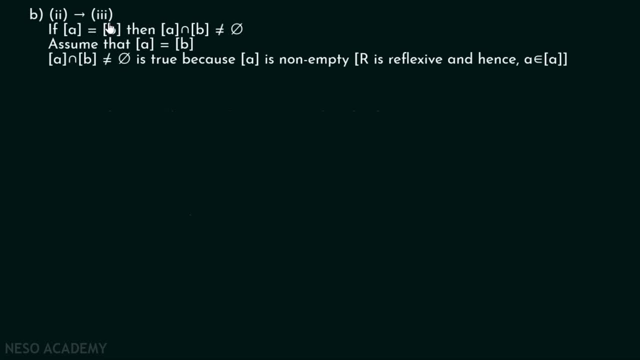 Now we will try to prove that 3 implies 1. This means equivalence class of A. intersection equivalence class of B not equal to phi implies equivalence class of A equal to equivalence class of B. Assume that equivalence class of A intersection equivalence class of B must not be equal to phi. 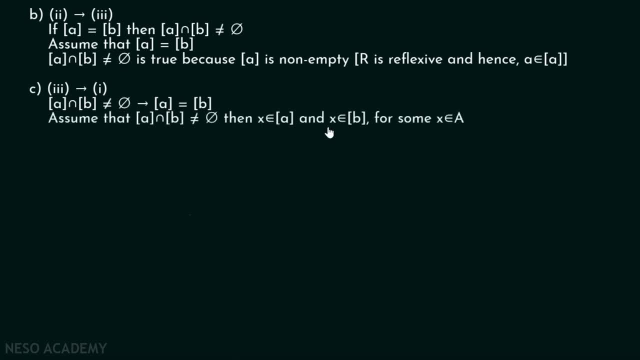 Then some x belong to equivalence class of A and the same x also belong to equivalence class of B. because intersection of these two equivalence classes is not phi Right, Let us assume that some element x belongs to both these equivalence classes. Okay, This x obviously belong to set A. 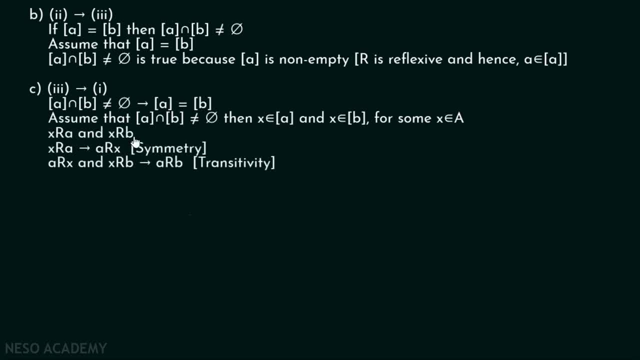 This means that x is related to A and x is related to B. According to symmetry property, if x is related to A, then A is related to x, Right, And if A is related to A, then A is related to B. 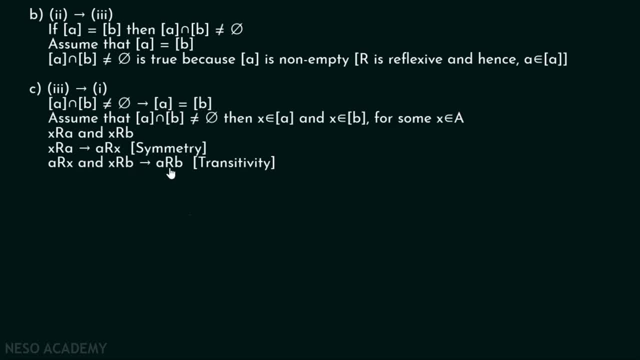 If x is related to x and x is related to B, then it means that A is related to B. This is according to transitive property. If A is related to B, then obviously equivalence class of A must be equal to equivalence class of B. 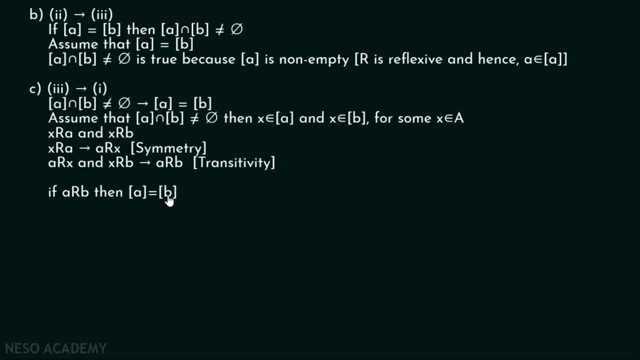 These two elements are related Right. Therefore they must belong to same equivalence class. Hence we can say that 1 implies 2, 2 implies 3 and 3 implies 1.. Therefore 1,, 2 and 3 are equivalent. 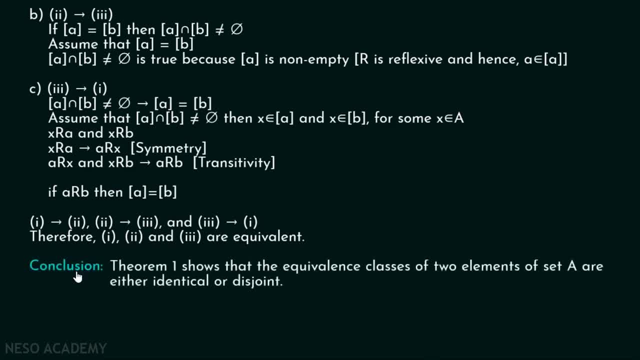 Now what is the conclusion of theorem 1?? Theorem 1 shows that the equivalence classes of two elements of set A are either identical or disjoint. We know that three statements are equivalent: A is related to B. Equivalence class of A equal to equivalence class of B. 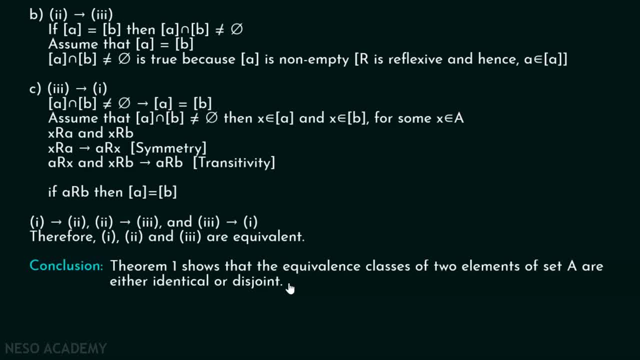 Apart from this, equivalence class of A intersection equivalence class of B must not be equal to phi Right. These three statements are equivalent. This means that when A is related to B, then equivalence class of A must be equal to equivalence class of B. 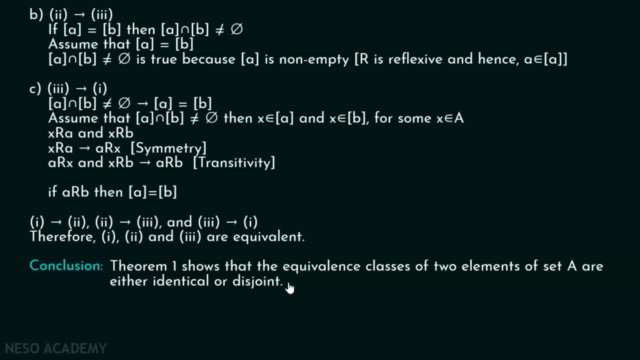 It must not be the case that they are different. Apart from this, the equivalence class of A intersection equivalence class of B must not be equal to phi, Which means that there are some common elements between A and B. This simply means that when A is related to B, then two equivalence classes must be identical. 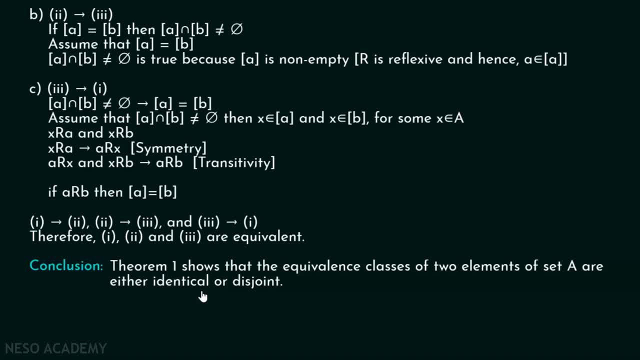 If A and B are not related to each other, then they must belong to different equivalence classes and they must be disjoint. There must not be any common element between those equivalence classes. Right? Therefore, it is clear that equivalence class of A- intersection equivalence class of B, must be equal to phi. 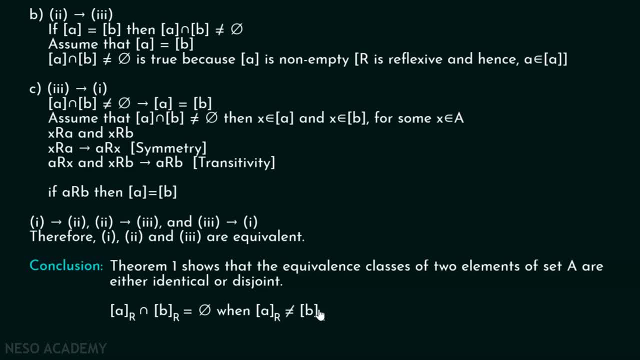 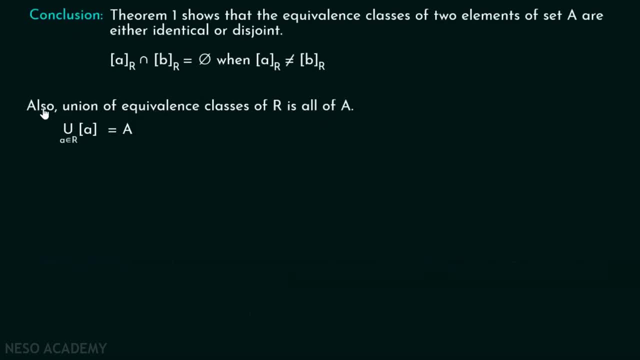 When equivalence class of A is not equal to equivalence class of B Right. This means these two equivalence classes are disjoint Right. Also, union of equivalence classes of R is all of A. Union of all equivalence classes must be equal to A. 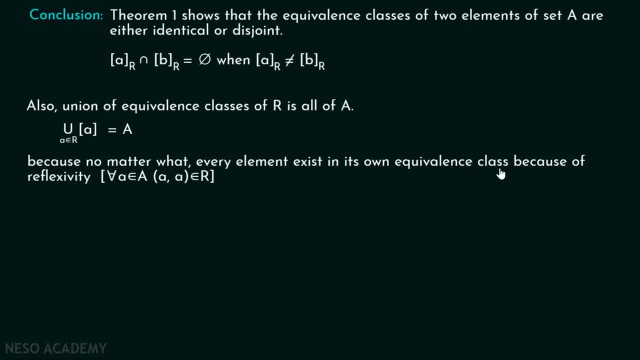 Because, no matter what, every element exists in its own equivalence class. because of reflexivity Right, Let's say we have set A, which consists of three elements: 1,, 2 and 3. In the worst case, they all belong to different equivalence classes. 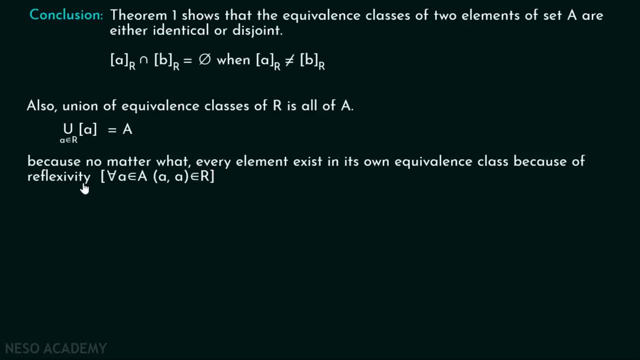 Right. 1 must belong to its own equivalence class, 2 must belong to its own equivalence class. 3 must belong to its own equivalence class And 3 must also belong to its own equivalence class. Right, Because 1 is always related to 1.. 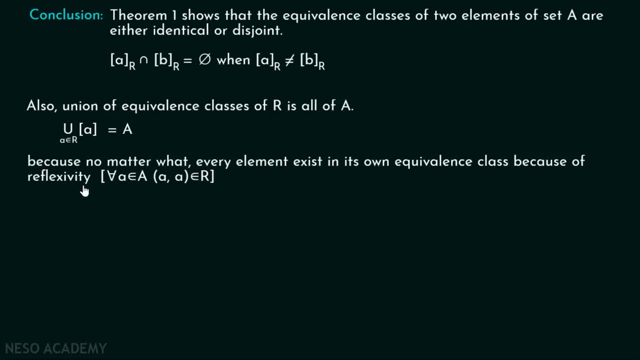 2 is always related to 2.. 3 is always related to 3.. This means, no matter what, every element exists in its own equivalence class Right. Therefore, union of all the equivalence classes must be equal to A, That is set A on which the relation R is defined. 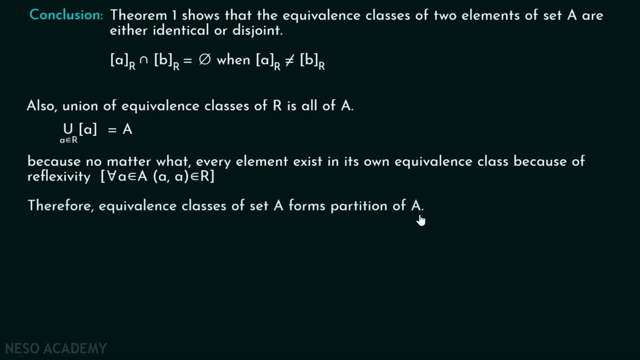 Therefore, equivalence classes of set A forms partition of A. This is very important to note. Equivalence classes of set A forms partition of A. What do we mean by partition? Partition of set A is a collection of all disjoint, non-empty subsets where I belongs to. I 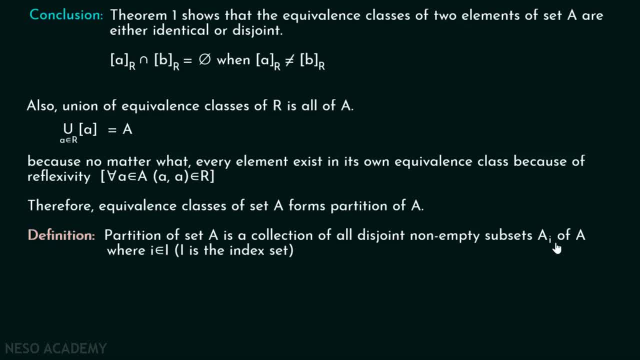 This I is the index set. I actually want to say A1, A2, A3 and so on. Okay, These are all subsets of set A. It must be well noted that AI must not be equal to phi, because they must be non-empty subsets. 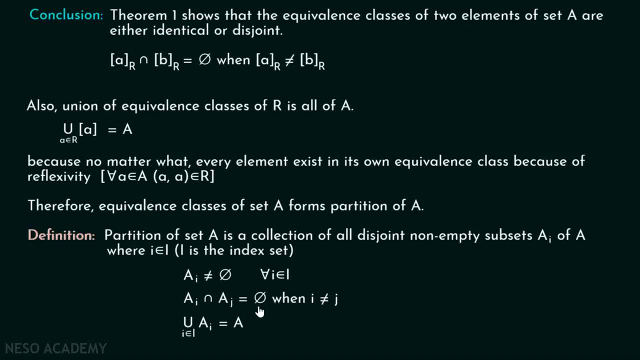 Apart from this AI intersection, AJ must be equal to phi. if I is not equal to J, Right. Their intersection must be equal to phi. They must be disjoint, Right. Apart from this, union of all the AIs will give me A. 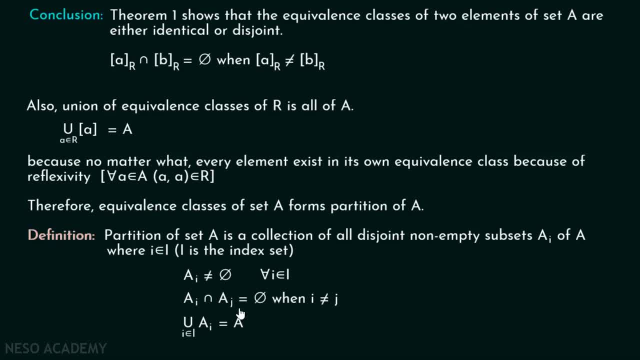 That is set A. This means that all the equivalence classes are equal to A. Equivalence classes of set A forms partition of set A. These subsets are actually dividing the set Right. Let's consider one example in order to cement the concept of partition. 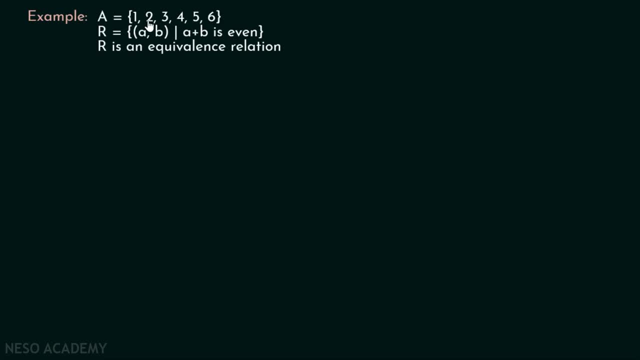 Let's say we have set A, which consists of these six elements: One, two, three, four, five, six- And we have relation R, which is defined on this set, Which is nothing but set of all ordered pairs such that A plus B is even. 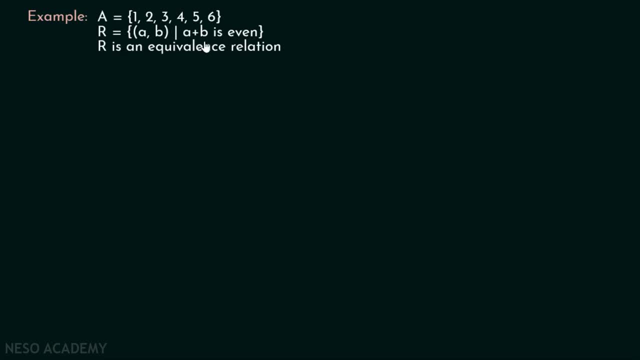 Okay, Now let me tell you: this relation is an equivalence relation. We already know this Right. Relation R is an equivalence relation. You can check this on your own. We have done this already. Right, We know that there are two equivalence classes which we can form from this relation. 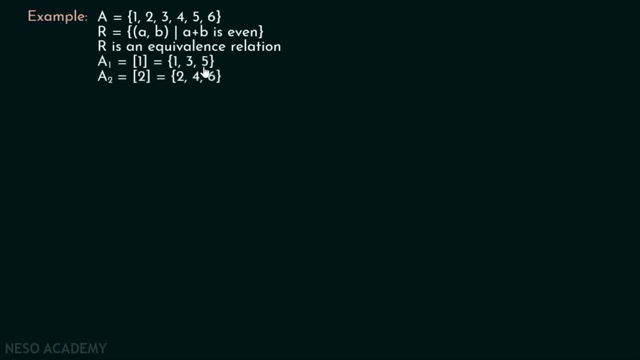 First is this equivalence class, one which is equal to one, three, five, And second is two, which is equal to two, four, six. Here, every element in this set is related to each other. Two is related to four, Four is related to six.